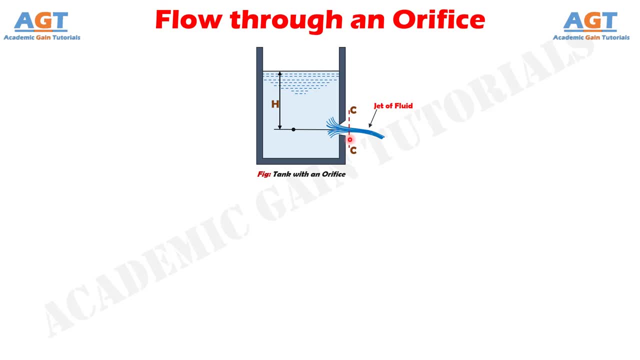 of diameter of the orifice. At this section the streamlines are straight and parallel to each other and perpendicular to the plane of the orifice. This section is called venecontractor. Beyond this section, the jet diverges and is attracted in the downward direction by the gravity. 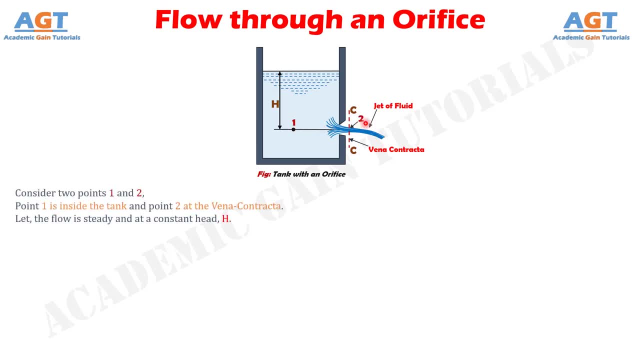 Consider two points, 1 and 2. as shown in this figure, Point 1 is inside the tank and point 2 is inside the tank. Point 1 is inside the tank and point 2 is inside the tank. Point 2 is at the venecontractor. Let's consider: the flow is steady and at a constant head. 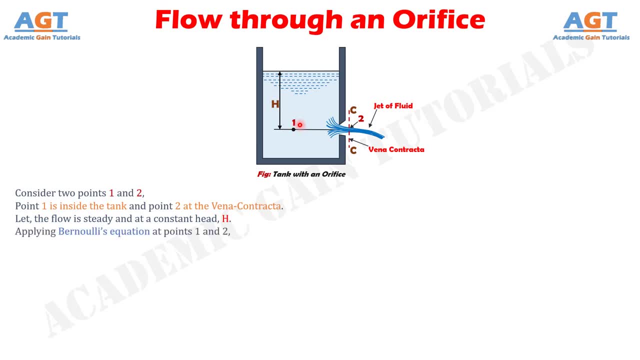 H. Now, applying Bernoulli's equation at points 1 and 2, we get P1 divided by rho g plus V1. square divided by twice g plus Z1 equals to P2 divided by rho g plus V2, square divided by twice g plus Z2.. But here Z1 and Z2 are equal. Therefore, deducting Z1, 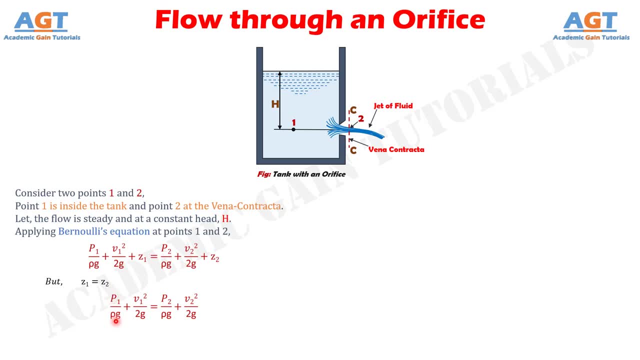 and Z2 from both sides. we have P1 divided by rho g plus V1 square divided by twice g equals to P2 divided by rho g plus V2 square divided by twice g. Now P1 divided by rho g will be equal to H. 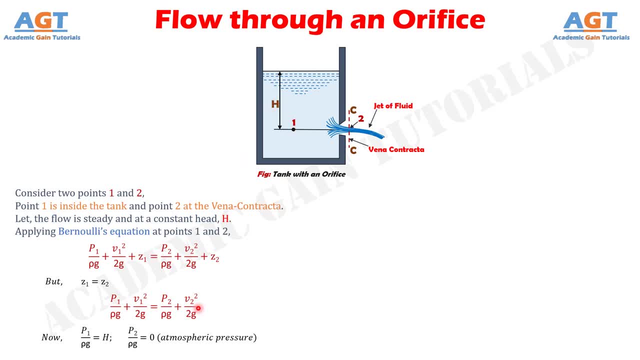 since it is inside the tank, And P2 divided by rho g will be equal to 0, since it is under atmospheric pressure. Again, V1 is very small or negligible in comparison to V2, as area of tank is very large as compared to. 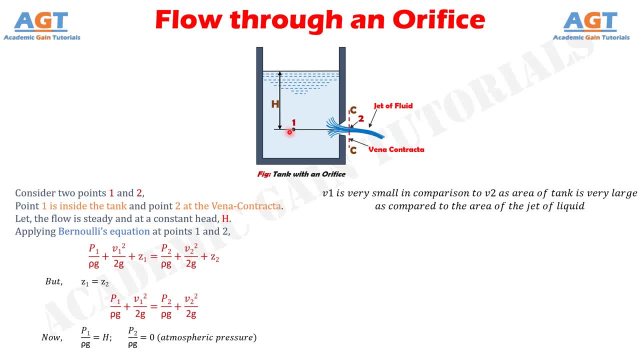 the area of the jet of liquid. So V1 can be considered as 0.. Now, putting the values in this equation, we get: H plus 0 equals to 0 plus V2 square divided by twice g. Now, solving this equation, we finally have velocity. V2 equals to root over 2 g H. This is theoretical. 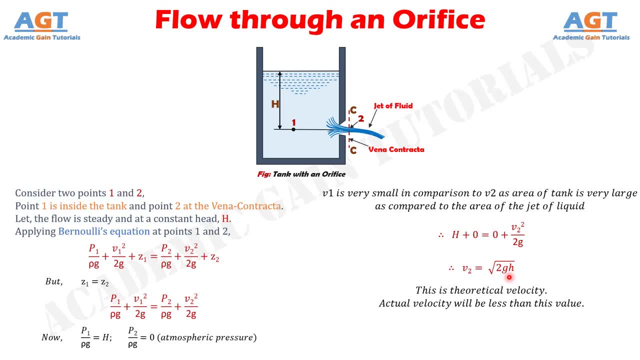 velocity. Actual velocity will be less than this value.